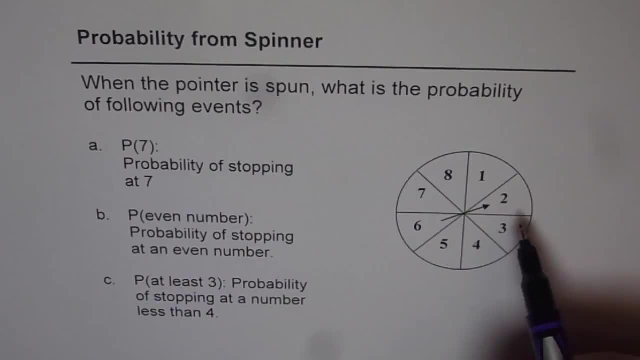 Now, in a spinning wheel- this one- we have 8 equal parts. That means when you spin this pointer it could stop at one of these places. So the total number of, or the possible number of outcomes is 8.. So we know number of outcomes. 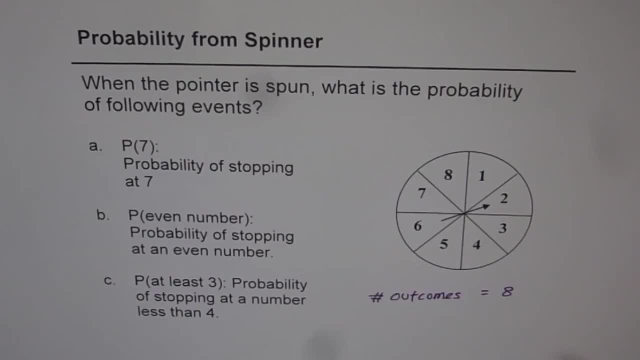 And that is 8 for one spin, right? So it could stop in 8 possible locations, And all are equally likely, since each portion is equal part, right. Now let's get back to part A, which is probability of stopping at 7.. Now, how many 7s are there? There is only one, 7,, right? So it is one favorable chance for probability of stopping at 7, and therefore P of 7.. 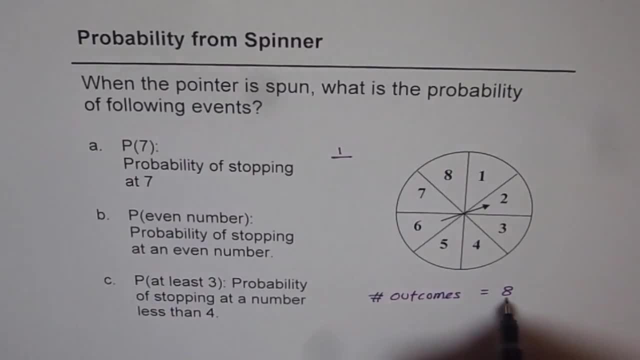 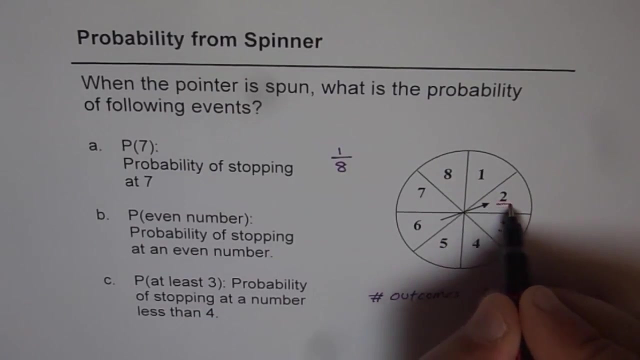 Now, what is the number of known course for probability of stopping at 8.. Now that we have to find out in this是這樣するian, fix it with the double stressed metric. we have to write down all the those points that we still have with this string expression: Two, four, six and eight. The golden number is 1 out of the total authenticity borrowing power from the third swelling parameter. So here I've got only 1,, 1 out of which is 8.. Thatumen of two pun restaurants will be 1, out of total number of outcomes, which is 8.. So the answer is 1 over 8,, right? The second one is probability of this pointer to stop at an even number. So how many even numbers do we have? As far as the even numbers are concerned, 2,, 4,, 6, and 8.. 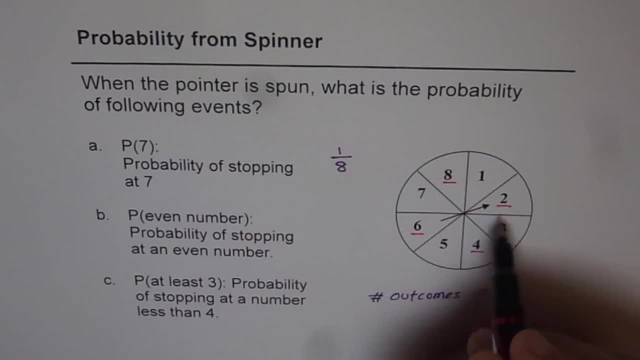 four even numbers. So if it stops at either one of these four, we get even number right. So favorable outcomes are four for us, four out of eight. So the probability is four out of eight, which could be written as half or 50% right. The last one is probability of stopping at a number. 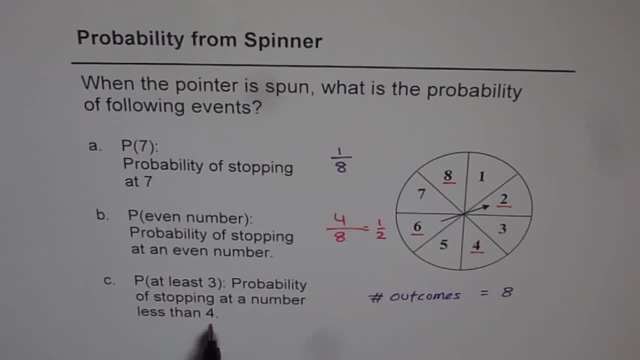 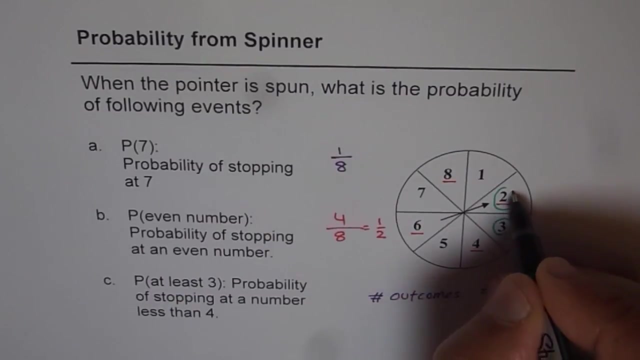 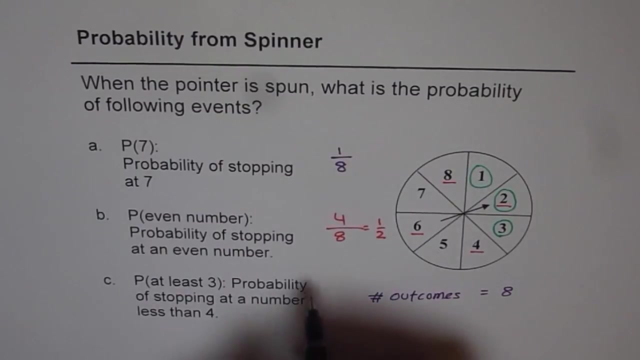 less than four, or we could also say probability of stopping at a number which is at least three. Now, how many of these numbers are less than four or are at least three? So we have three, two and one. So there are three numbers which are at least three out of eight. And therefore,